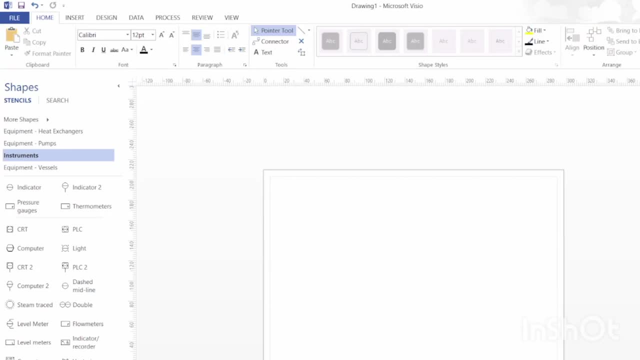 For this purpose I will just google and copy paste any diagram in standard pft. I will paste it here and we will follow steps to draw the diagram In this pft. we have a CSTR that is connected with the wells and pipeline. 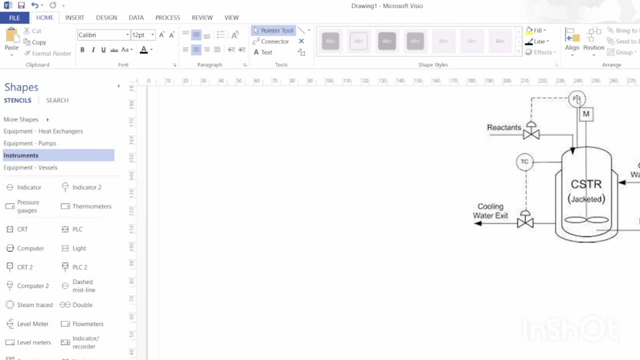 This pft also includes the indicator. First we will go to the vessels. Before that, I would mention that the shapes can be selected from the engineering. I have already told you that for campaign engineering we use process engineering instruments that I have already selected. 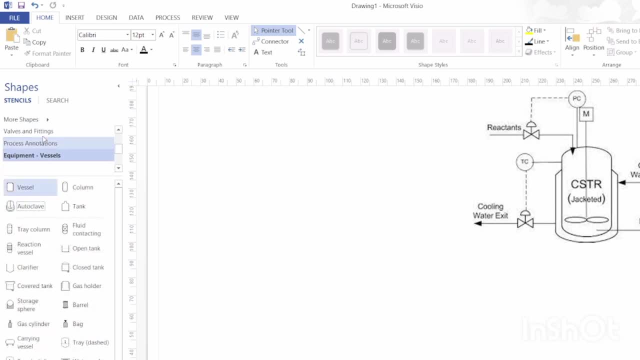 Thank you. I will go to the vessels and draw a CSTR. After that I will draw a pipeline. I have already told you that the shapes can be selected from the engineering. After that, I will go to the vessels and draw a pipeline. 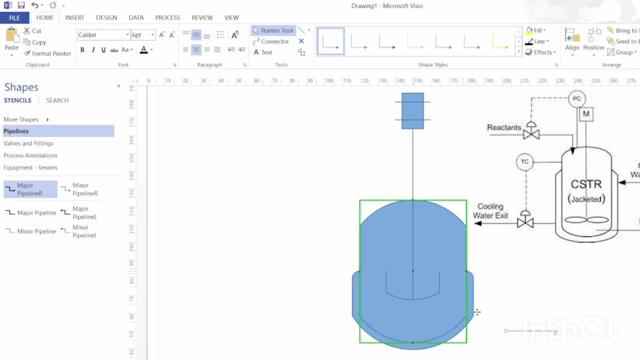 After that I will draw a pipeline. For these diagrams. I will just go for major pipelines For these diagrams. I will just go for major pipelines. After that I will draw a pipeline. It is connected with a valve. We have a diaphragm valve here, so I will just plug it here. a diaphragm valve and then again the piping. 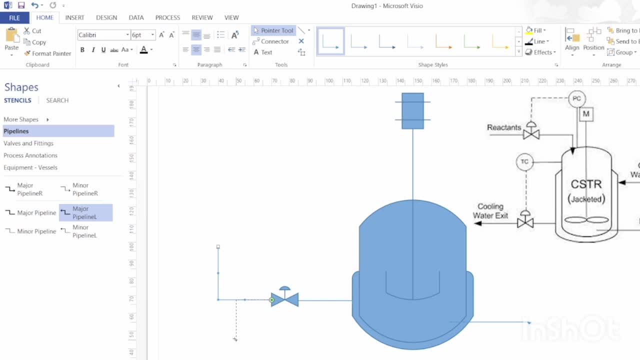 Okay, this valve is connected with an indicator that will be found in the instrumentation section. Okay, we have different kinds of instruments and indicators. It is connected with a signal. We have a signal with a valve, which is also connected with a CSTR. 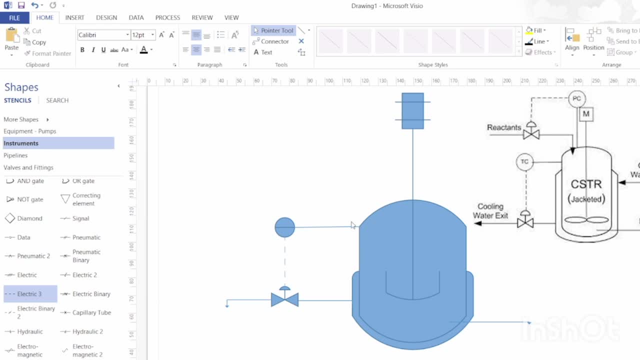 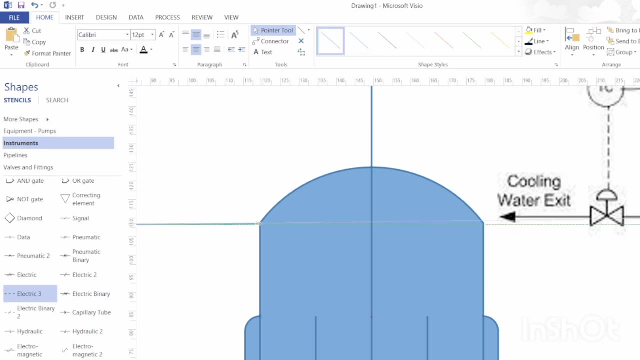 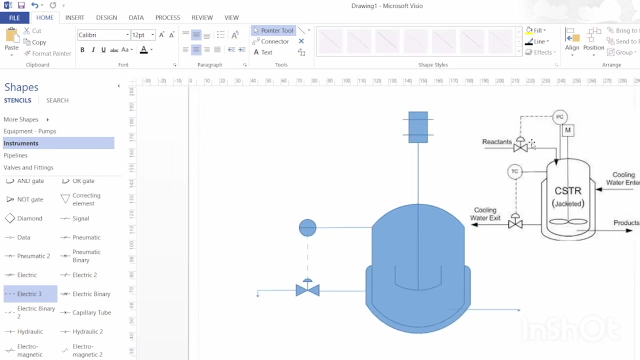 It is very nice. It is very important to make sure the line is straight. After that, we have another valve. I will just copy-paste that valve on here- And then we have a pipeline. Okay, so we just find out that the pipeline you are controlling needs to be the CSTR for us. 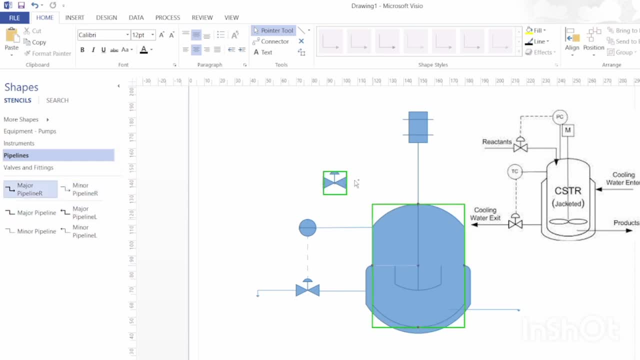 so we just have an indicator out of thatабатic so that we can do whatever we want with the sensor. So the first thing we want to do is test To see what is still left over from the diagnostics curl when we get continues. 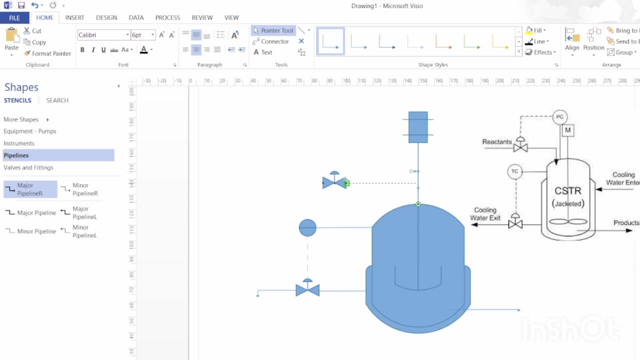 because our students an they send us information about whether this was the best 잘gh domain of measurement, And so we focus on identifying this as well as as to knowing whether this is correct or not. Thank you, Thank you, Thank you. 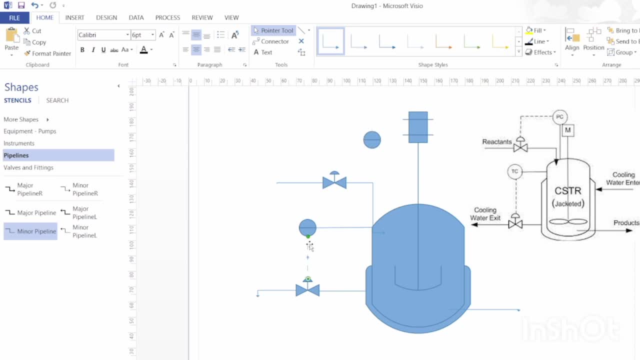 And end by selecting what's currently. there is no need, So we are left with a good note And it is entering the circuit. So the diagram is almost complete. I will just select it and then change the color. We can color it according to our choice. 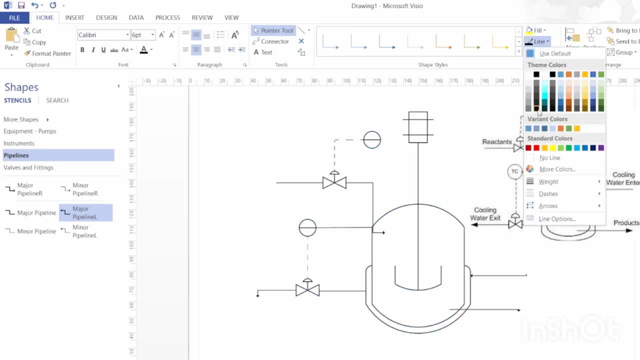 but I am not curving it. I am just changing the color of the line to black and also the thickness to 1.5.. Now you can see there is one confusion here, So that's why I will just make it clear That line also needs. 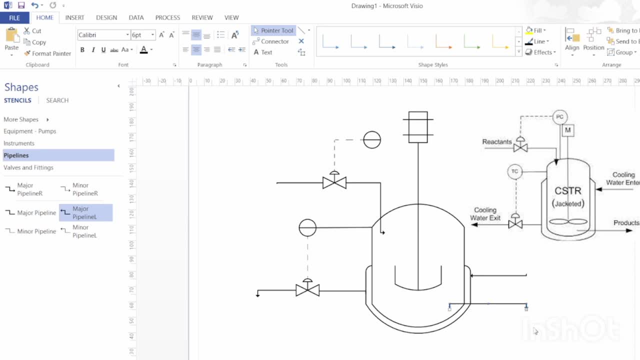 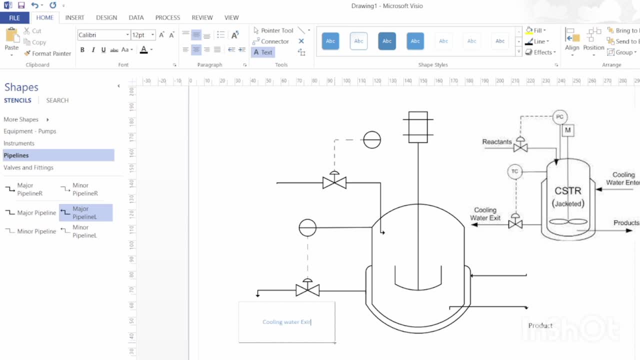 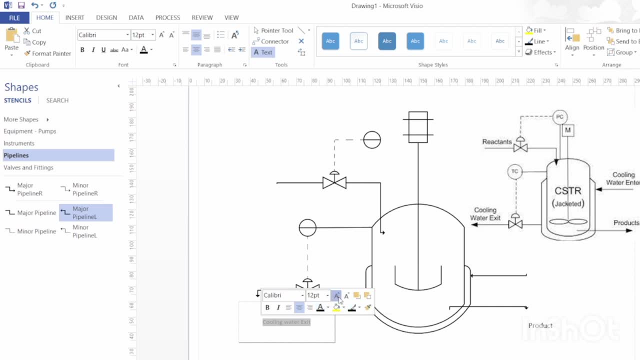 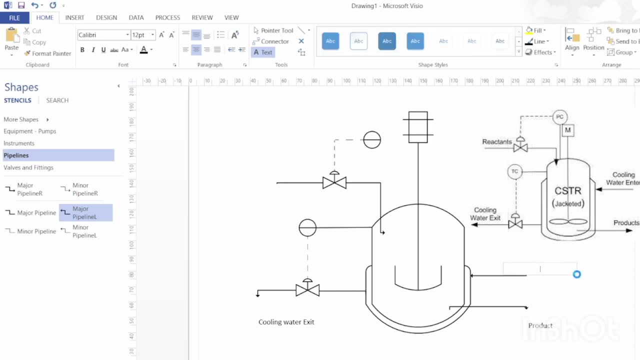 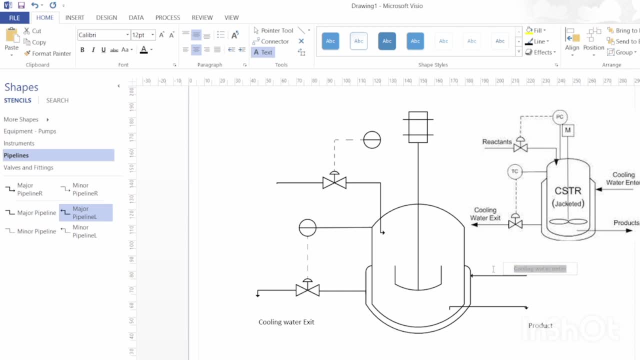 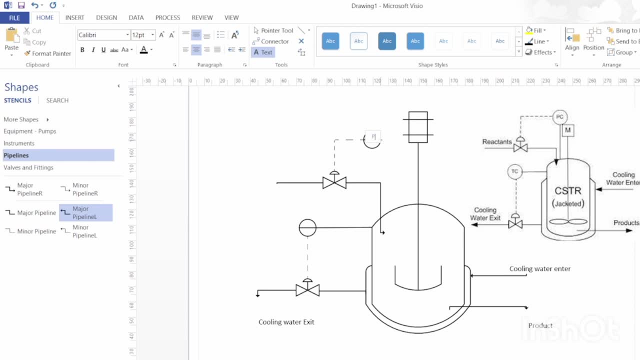 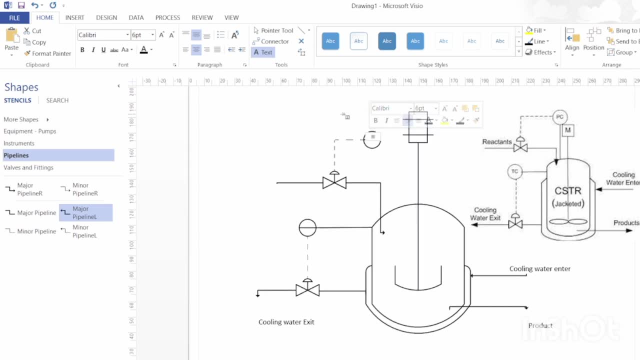 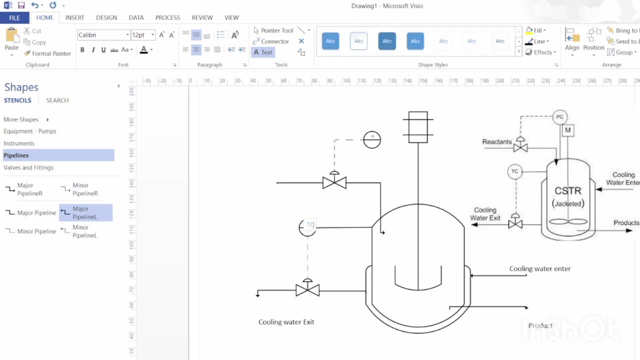 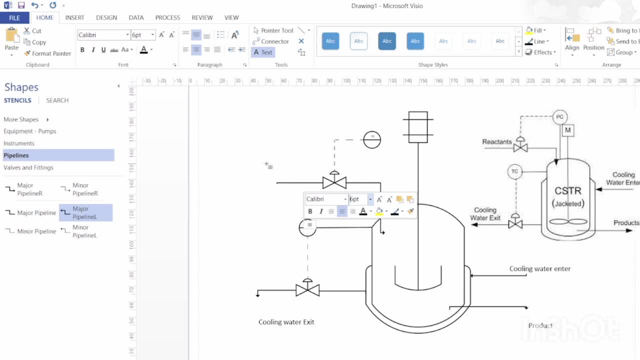 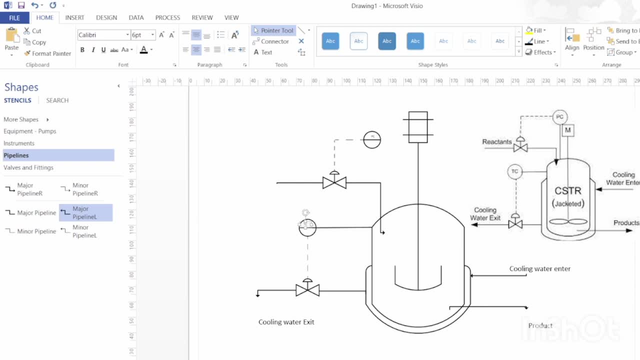 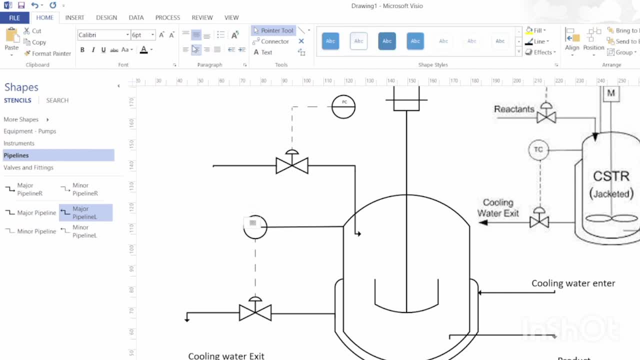 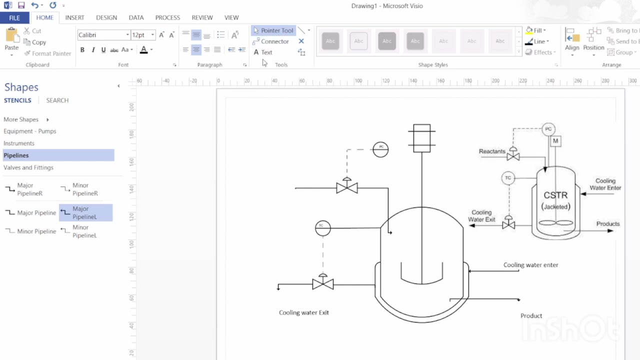 You can also change the font size. The other holders were done, that is to say, changing the color of the form to the size So that you can clearly see. Okay, now you can see. the diagram is complete. I haven't mentioned the CSTR here. 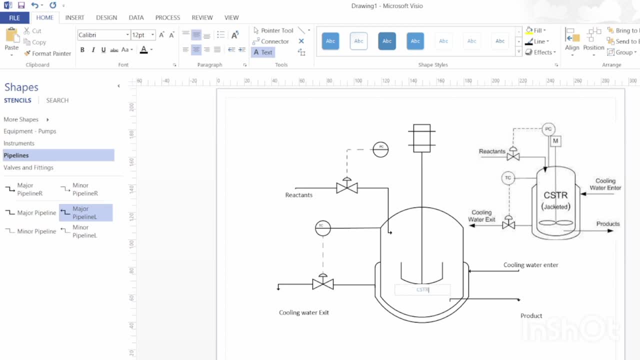 Okay, CSTR And change the color size and make it prominent. You can also save the files, And we have just deleted the picture, So the diagram is complete. Thank you, and keep watching for more.